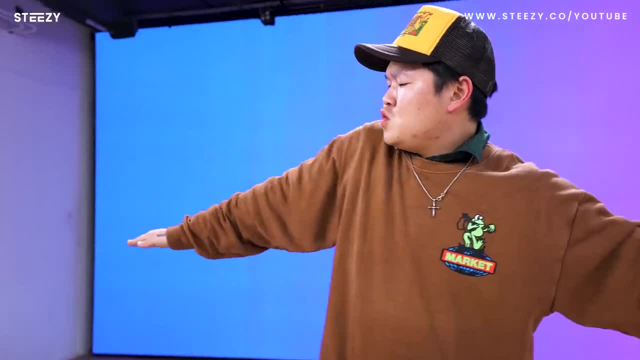 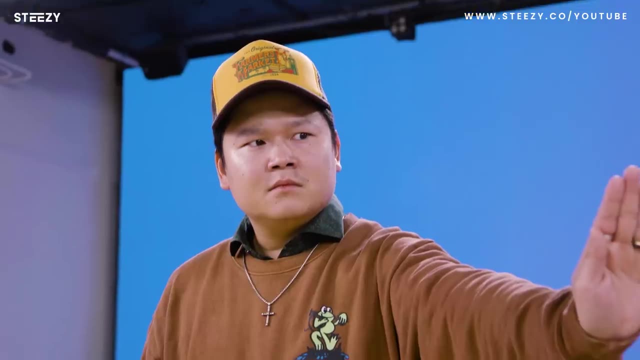 We'll start with a four-point arm wave, then we'll learn a six-point arm wave. You'll see what I mean. The simpler four-point arm wave starts with raising the hand like you're telling someone to stop. Then you relax your hand and raise your wrist like you're a praying mantis. 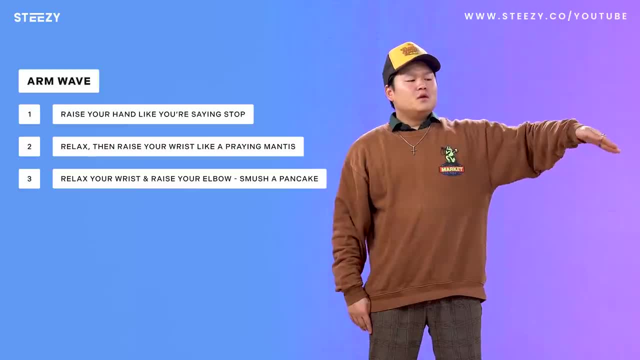 Then the hardest step: relax your wrist and raise your elbow. You should look like you're smushing a pancake or something. Then straighten your arm and raise your arm like you're a praying mantis. Raise your shoulder to your ear. 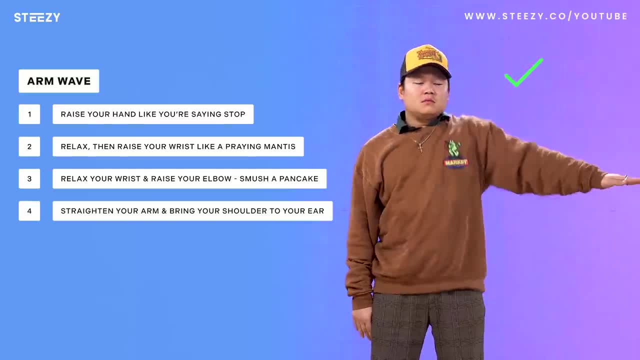 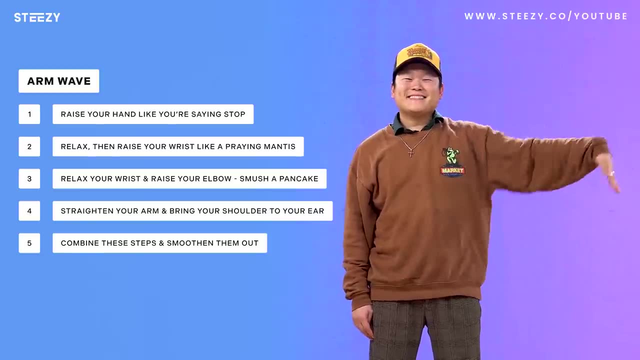 Do not bring your ear to your shoulder. Combine those steps, smooth them out and even reverse it, with no stops between each segment, to get a smooth arm wave. Now we'll do the much cooler, much more handsome-looking six-point arm wave. 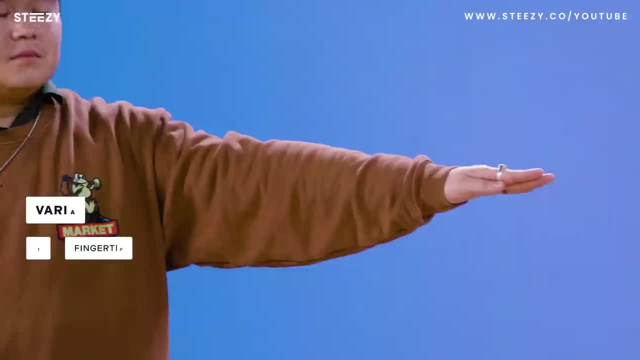 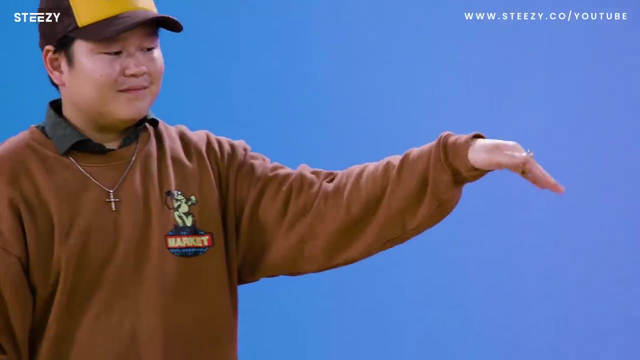 which has all the same steps, except you add a few points to the beginning: The fingertips lifting The minor knuckles, lifting The major knuckles, Then continue into the same steps as before, with the praying mantis, the smushing pancake and the shoulder raise. 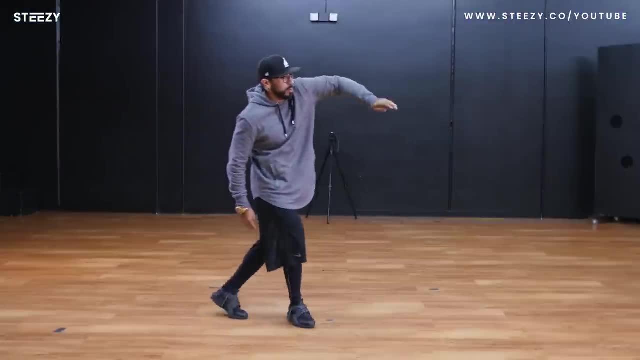 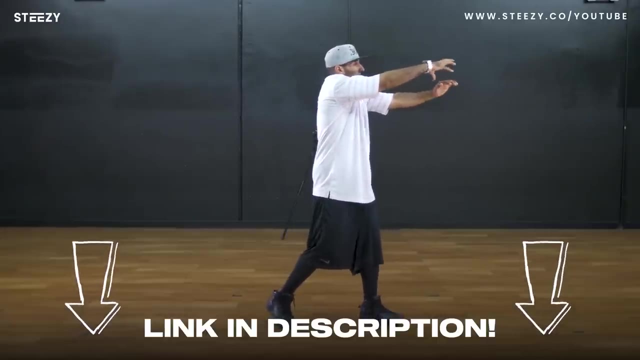 If you want more detailed lessons on waves, from beginner all the way to really freaking advanced, you should check out Boogie Frantic's waving classes on STEEZY. Those classes actually changed my life and helped me understand waving on a level that I never knew existed. 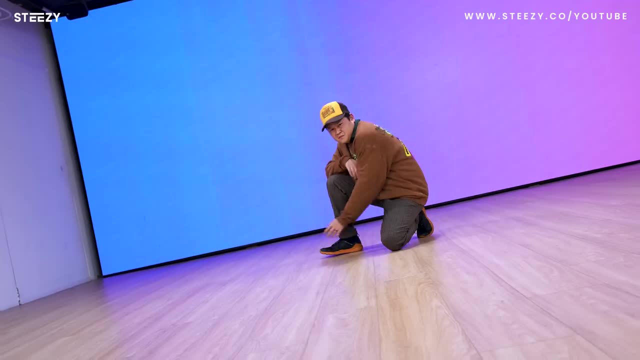 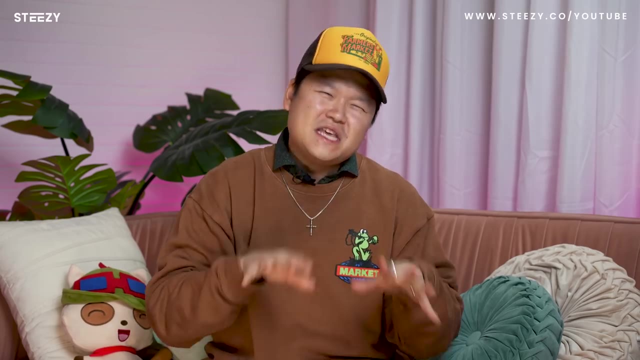 Move number three: the knee slide. This is such a simple yet effective move to cover ground at the beginning, middle or end of a dance. It's confident and it's sexy. Also, don't be afraid to wear knee pads as you practice this and learn how to do it correctly. 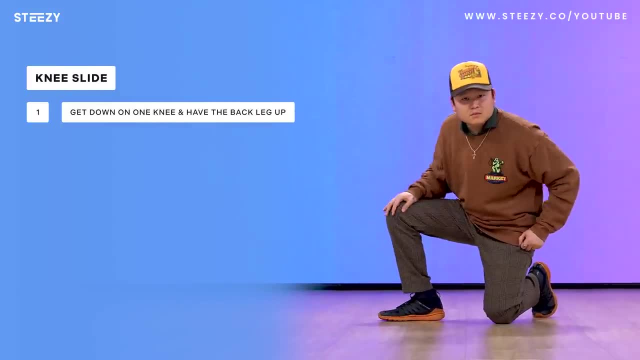 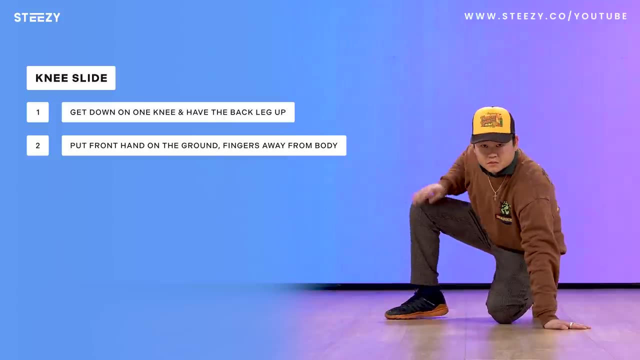 Get down on one knee and have the back leg up like this. Put your front hand on the ground and face the fingers away from the body. You don't want them to face inwards. Use your back leg to push yourself forward off the ground while your rested leg swings forward. 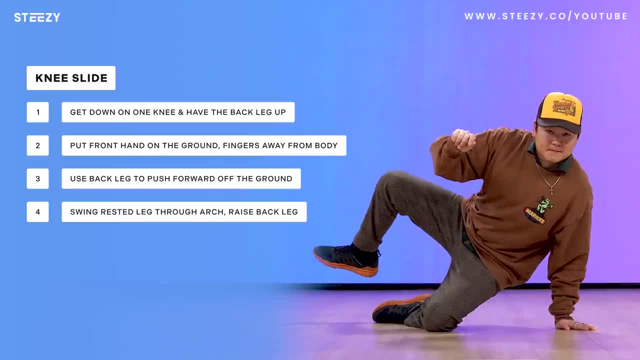 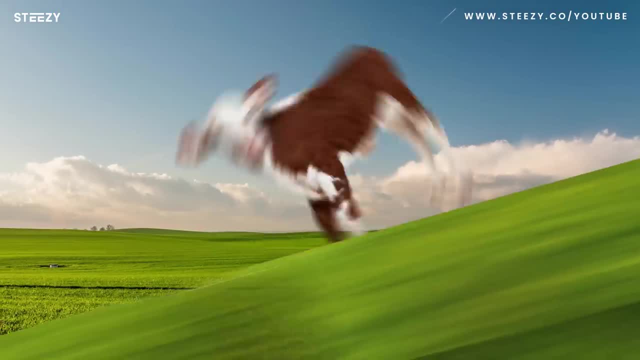 through the back leg's arch and slightly raise your back leg, You will actually be sliding on the side of your calf, even though the move is called a knee slide, because a calf slide sounds like a baby cow going down a hill. Finish your move by landing the raised leg's foot down and resting your arm on it. 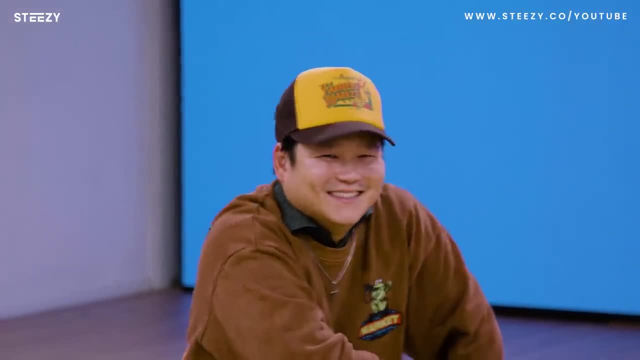 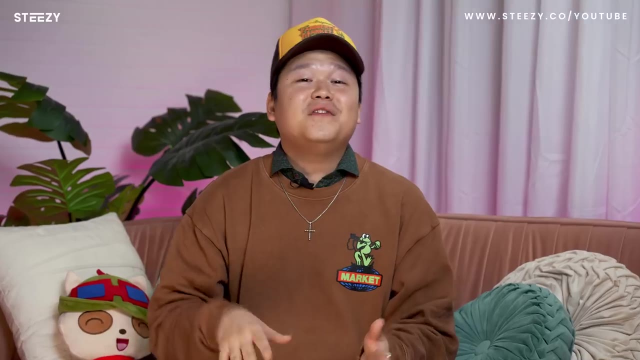 because it looks cool And you're cool. Move number four: scribble foot. This move is basically a faster, more grounded house version of a pas de bourrée. I didn't need to do that in the French accent, that was weird. 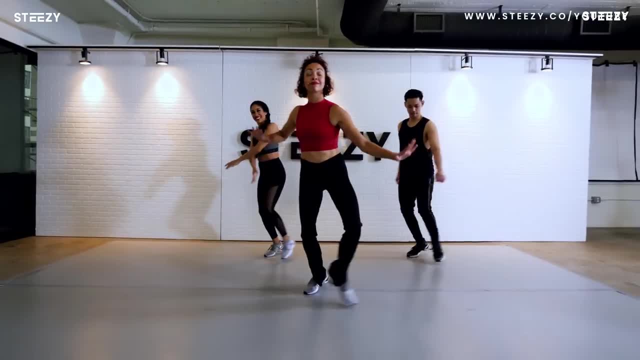 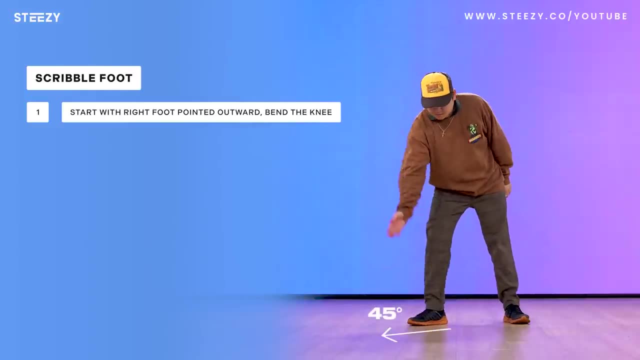 A pas de bourrée, which you'll see often in ballet or jazz dance, but it originated from ballet. Start with your right foot stepped out with the toes pointed 45 degrees outwards and bend the knees. then lean your weight onto it. 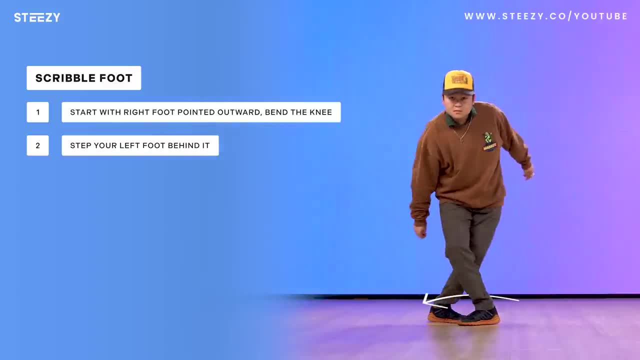 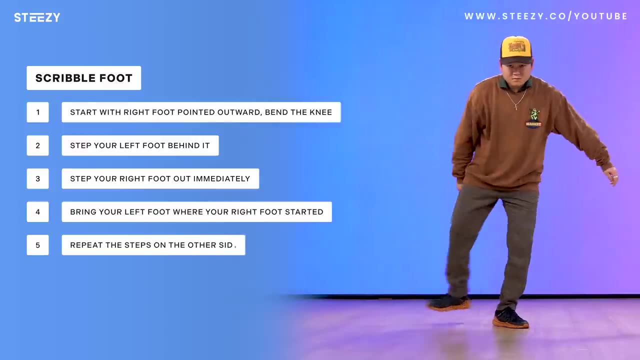 Step your left foot behind so it peeks past the right foot. Then step your right foot out immediately after And bring your left foot to the initial position your right was in. Repeat the steps on the other side. Then you want to speed up the move. 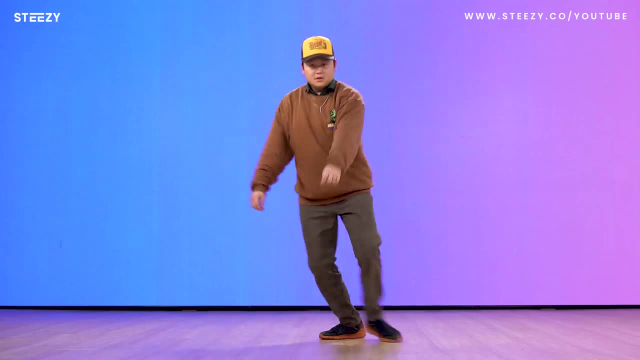 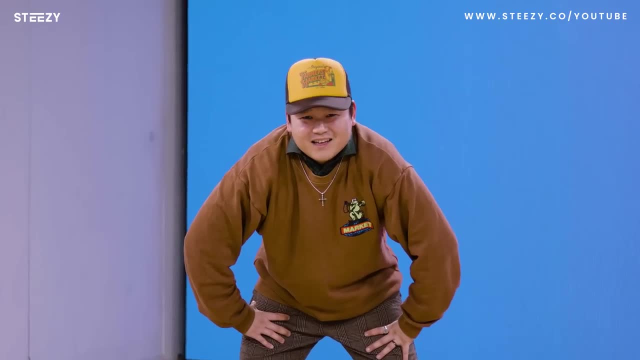 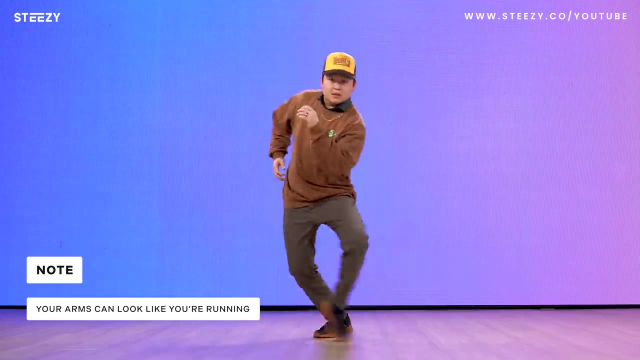 six E and seven E, and you know I can't even say it, but your feet will move fast. Your arms can be outwards and floaty or like they're running or crazy turning arms. Okay, no, just kidding, Don't do it. 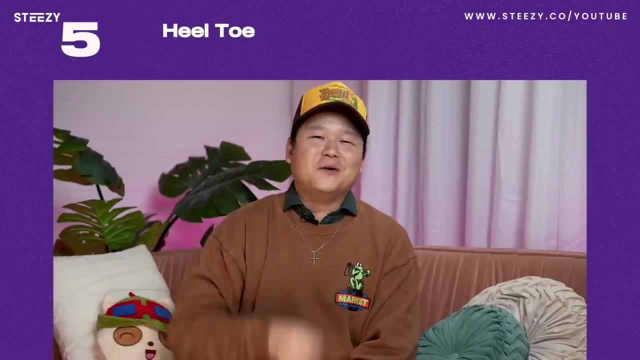 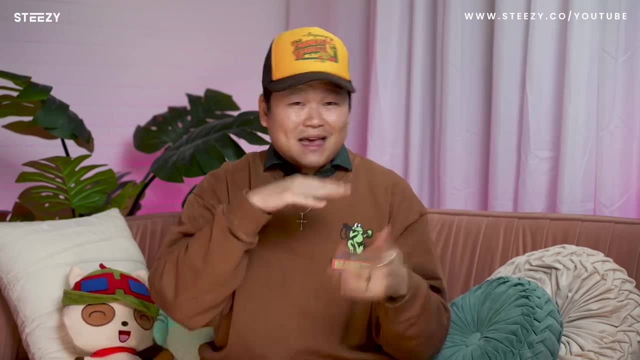 But are you down though? Move number five, the heel toe or V-step, or Mike and Ike or Pac-Man or Happy Feet? Okay, a disclaimer: Move names get wildly mixed up and switched up when it comes to social dances, And that is a beautiful yet terribly difficult thing to track. 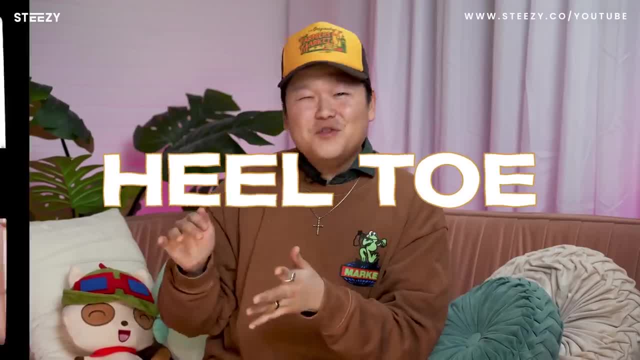 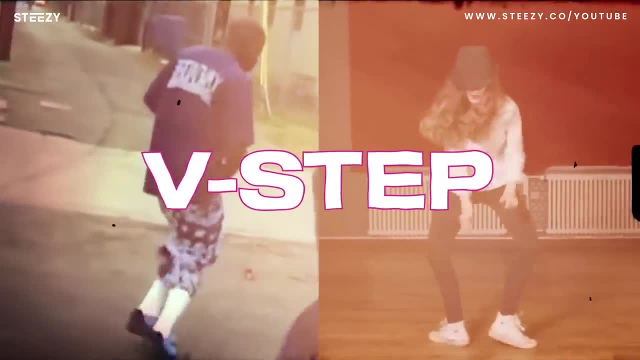 This move is sometimes called a heel toe, even though there's another move called a heel toe in house dance and hip hop. In sea walking and swing dance it's called a V-step And in the northeast of the US it's called a Pac-Man or Happy Feet. 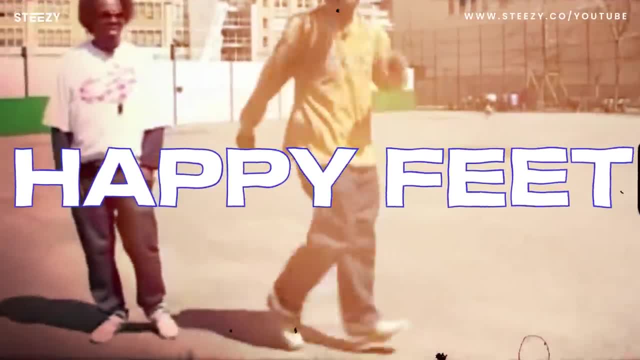 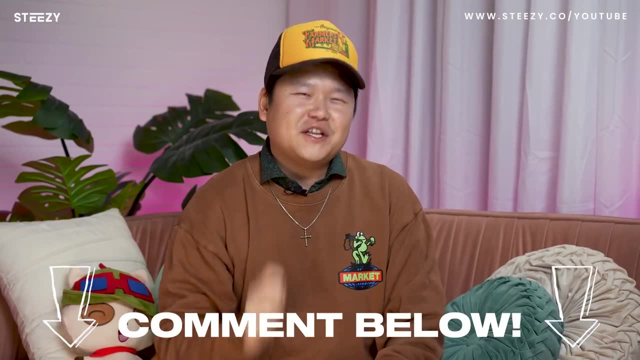 Even though the Happy Feet is also the name of this hip hop move And in Chicago it's called Mikes or Mike and Ikes, I digress. What did you grow up calling this move? Leave your answer in the comments. Let's practice this move sitting down to start. 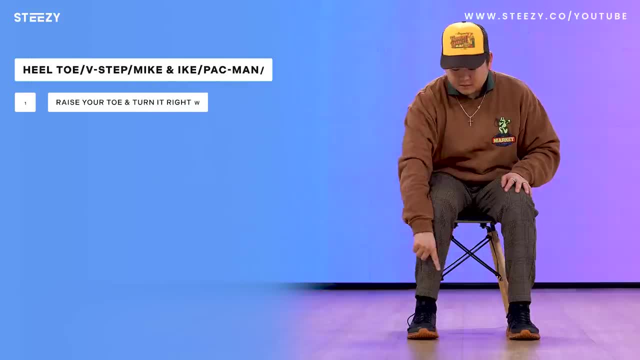 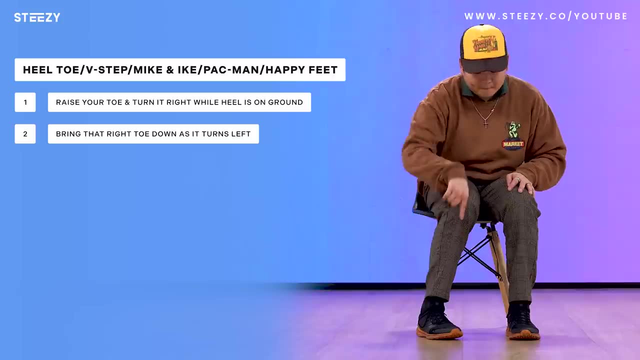 We'll do one foot at a time, starting with your right. Raise your toe and turn it to the right while your heel is on the ground. Bring that right toe down. Toe down as it turns left. Plant that toe and raise the heel to the left. 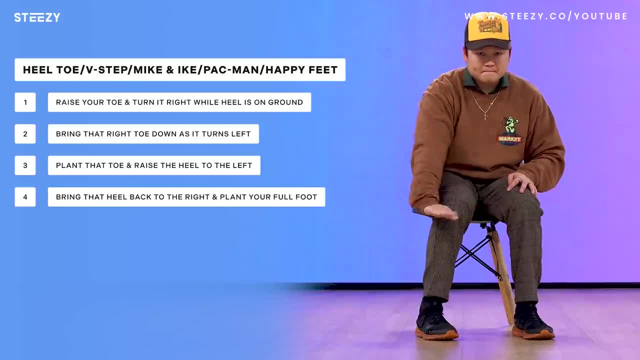 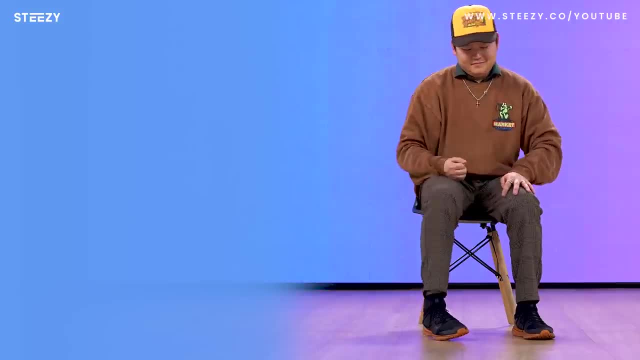 Bring the heel back to the right and plant your full foot. So toe down, heel down, Toe down, heel down. On the left foot, we'll raise our heel up and to the right, Heel down and to the left.